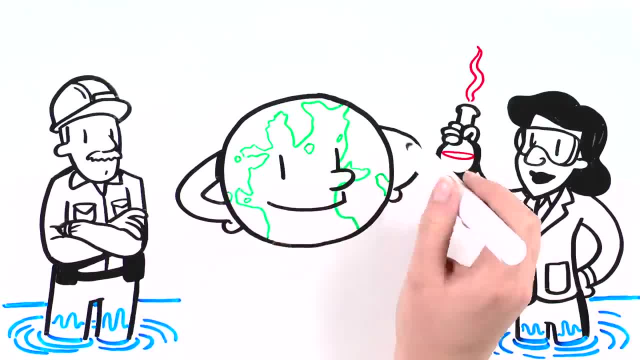 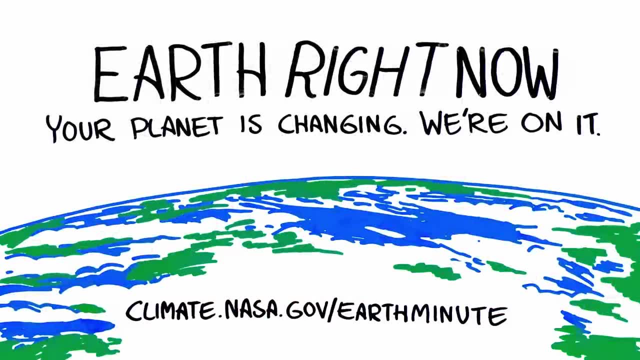 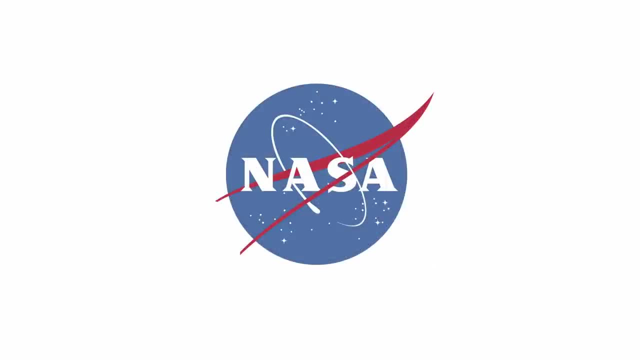 because right now good old Earth is the only planet we've got. NASA Jet Propulsion Laboratory, California Institute of Technology. 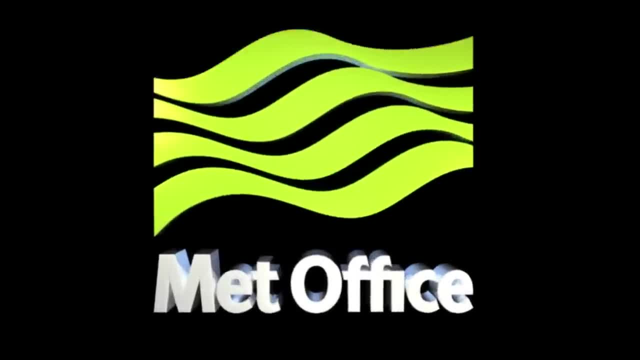 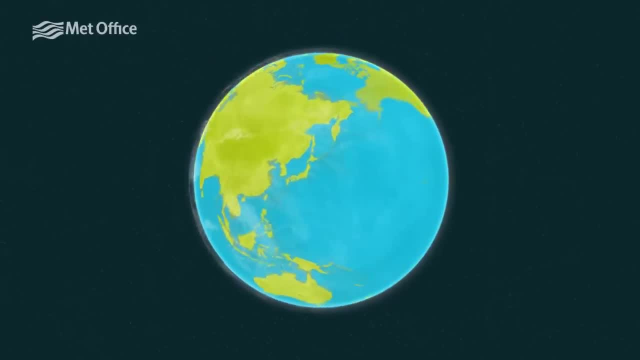 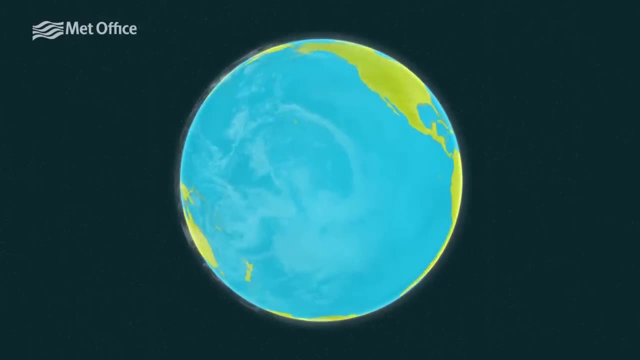 Every few years, the El Niño phenomenon kicks into life in the Pacific Ocean around the equator. It can affect weather around the world, changing the odds of floods, drought, heat waves and cold seasons for different regions, even raising global temperatures. 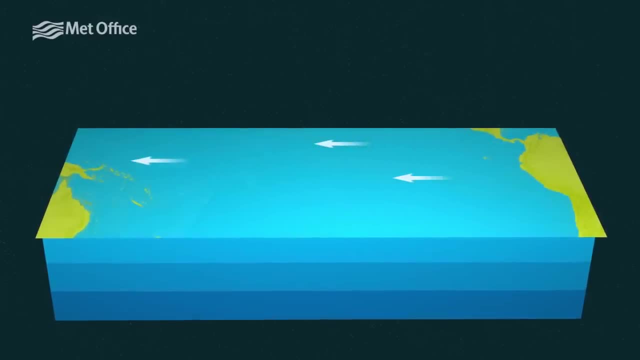 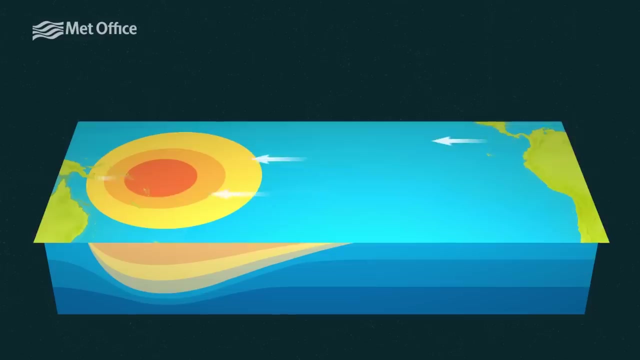 But what is El Niño and how does it happen? Firstly, we need to know what's normally happening in the tropical Pacific. This vast stretch of ocean sees consistent winds, called trade winds, that blow from east to west. These winds push warm water near the surface in their direction of travel, so the warm water piles up on the western side of the ocean, around Asia and Australasia. 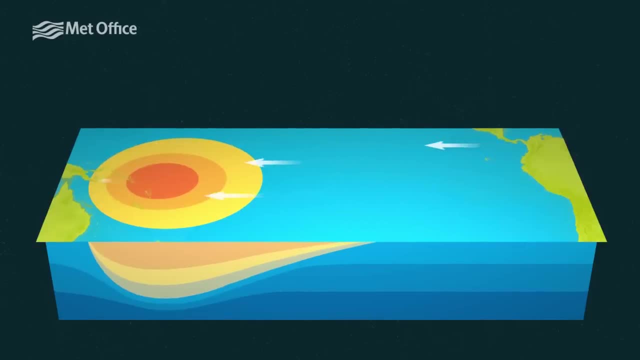 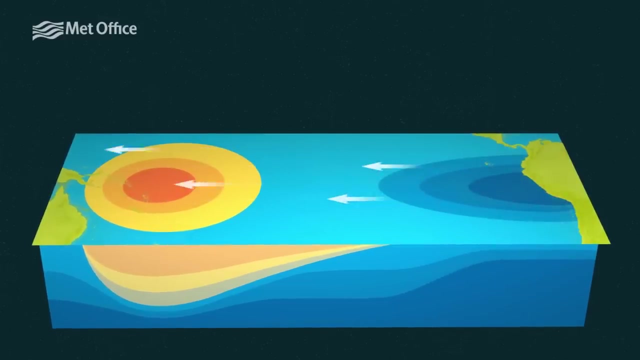 On the other side of the ocean, around South and Central America. as the warmer water gets pushed away from the coast, it's replaced by cold water which is pulled up from deeper waters. This creates a temperature difference across the tropical Pacific, with warmer water piled up in the west and cooler water in the east. 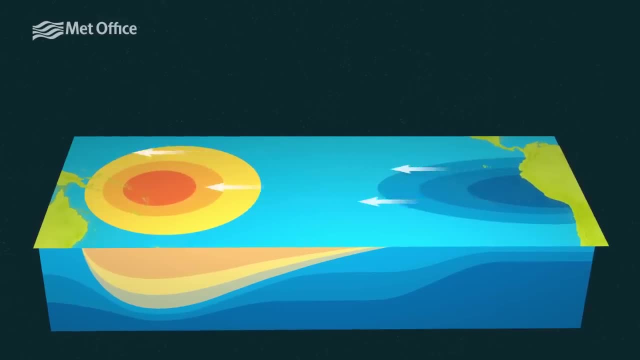 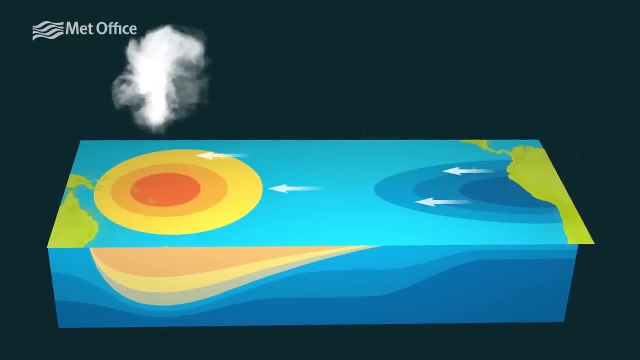 Warmer water adds extra heat to the air, which causes the air to rise with more vigour, and it's this rising air that creates an area of more unsettled weather, with more cloud and rainfall. That rising air in the west sets up atmospheric surveys. 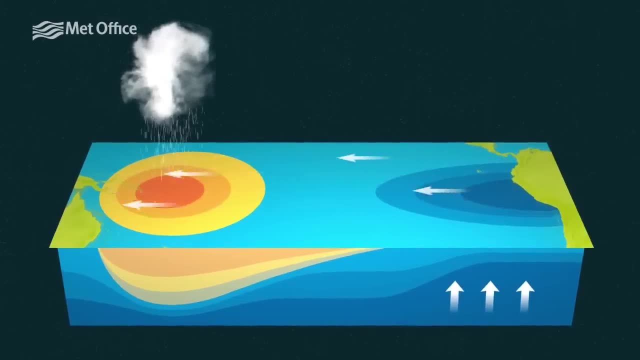 In the east. there's a lot of air circulation across this part of the world, with warm, moist air rising on one side of the ocean and cooler, drier air descending on the other. This circulation reinforces the easterly winds, so this part of the world sits in a self-perpetuating state until El Niño begins.